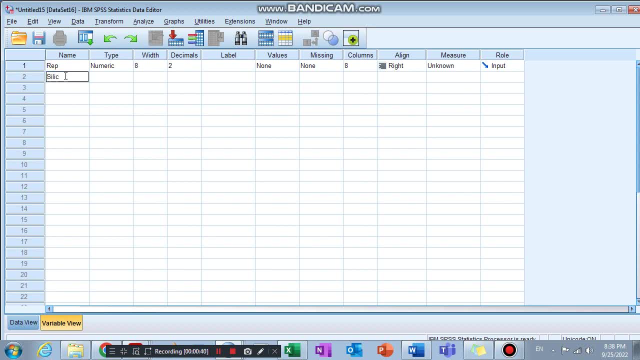 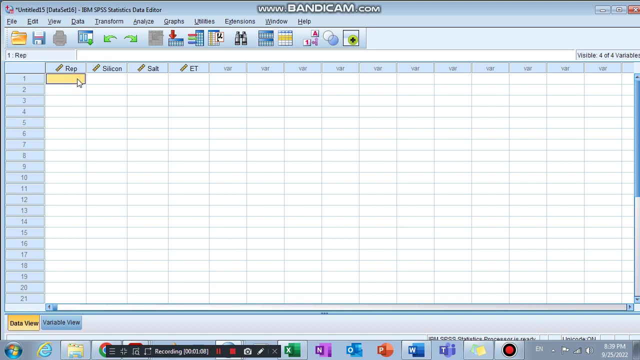 first factor of our experiments, silicon, the second one, salts, and we have two factors, silicon and salts. and the third one. we have this dependent variable, which is the transpiration of the crop. we have a field experiment, agriculture, field experiment- so we can represent our data here. so we have three replications for 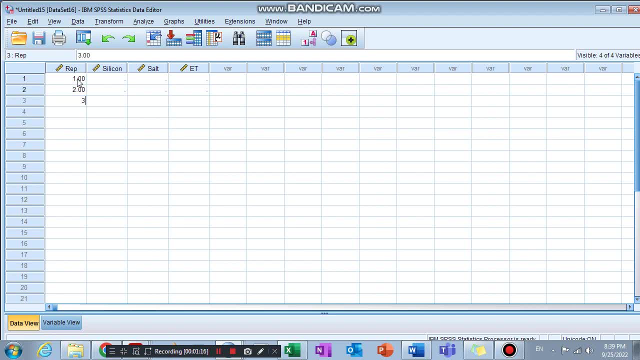 our field experiment: one, two, three, four silicon. we have three levels of silicon. the first level has to be in each replication. the second level of silicon: the second level has to be in each replication. the second level of has to be in each application. the search level. we have three replication each one. 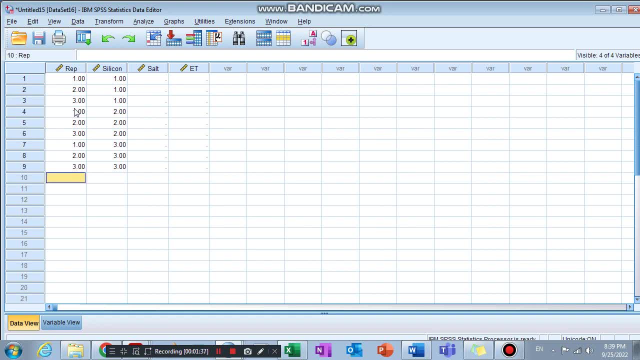 two, three, then salt. we have four levels of salts in our experiment, so one just. we have to make sure that each salts label has to be in each silicon level so that we can write the first level of salts here, then the second one, three, silicon, three, replication. we have nine salt label. I mean we have four level of salts. 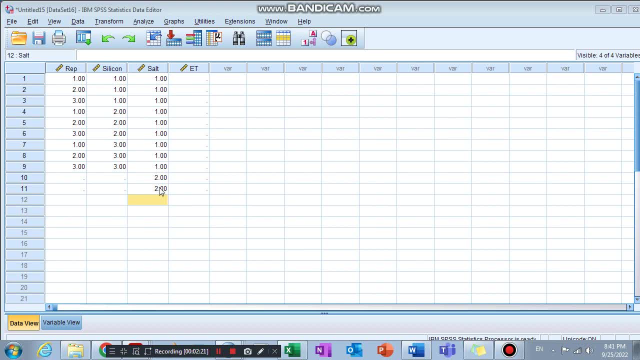 which has to be each level, has to be in each silicon level. so two, two, two, two, two, nine times because we have three, three application and three silicon. so three by three, nine. two, one, two, three, four, five, six, seven, eight, nine. so we have our application here. silicon levels: three silicon levels. salt level: we have four salt. 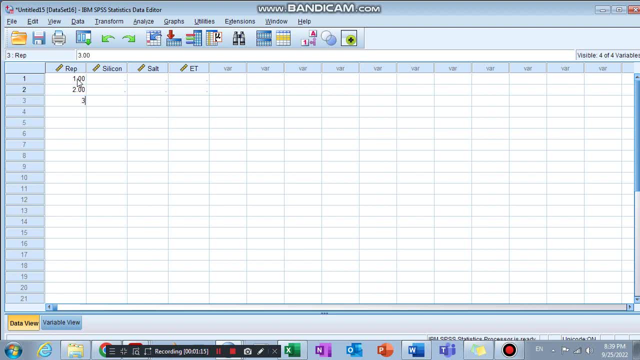 our field experiment: one, two, three. for silicon, we have three levels of silicon. the first level has to be in each application. the second level of silicon and the second level has to be in the second level of the second level has to be in each application. the search level. we have three replication each one. 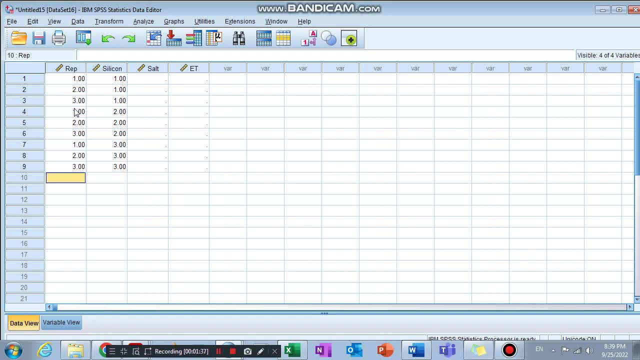 two, three, then salt. we have four levels of salts in our experiment, so one just. we have to make sure that each salt slave has to be in each silicon level so that we can raise the first level of salts, getting the second when three silicon tree application. we have nine. 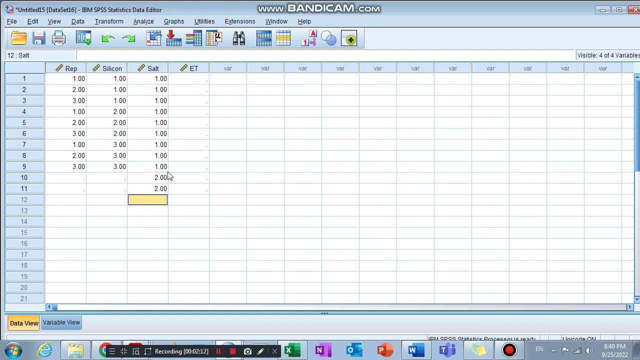 salt labor. I mean we have four level of salts which has to be. each level has to be in slicer function and the ils first level has to be in Fam. we are, i 감 2020. there is only a select welcome to to open a new folder. they let us go with that. we already have a score, we already consider. cool. i think we have, because i think you can open one of these. yes, Ça Te Print. So this in the os three, we have to be our I, why we got in the document. there are two Hyungers who have written a folder in the 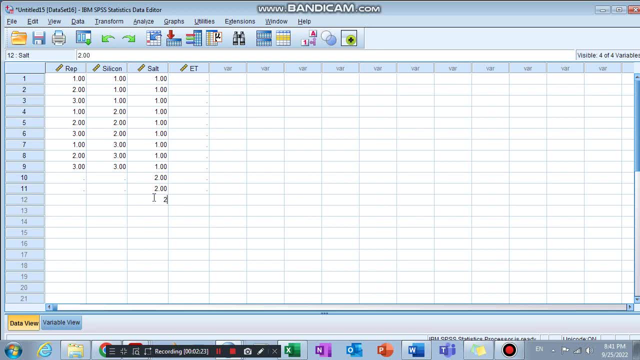 each silicon level. so two, two, two, two, two, nine times, because we have three and three replication and three silicon, so three by three, nine. two, one, two, three, four, five, six, seven, eight, nine, so uh, we have, uh, our replication here, silicon levels, three silicon levels, uh, salt. 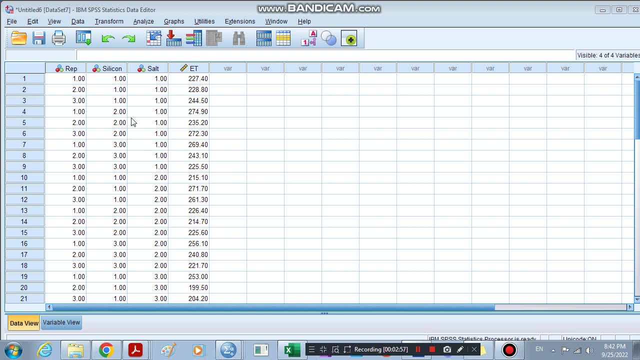 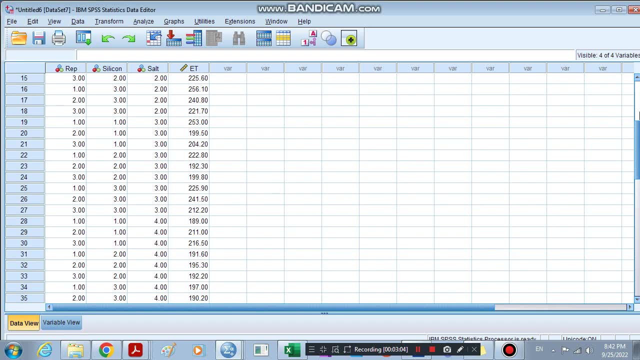 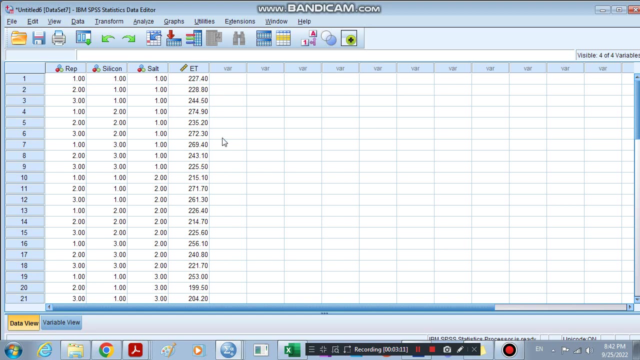 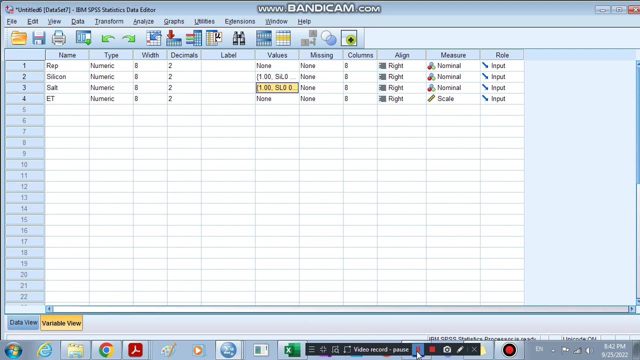 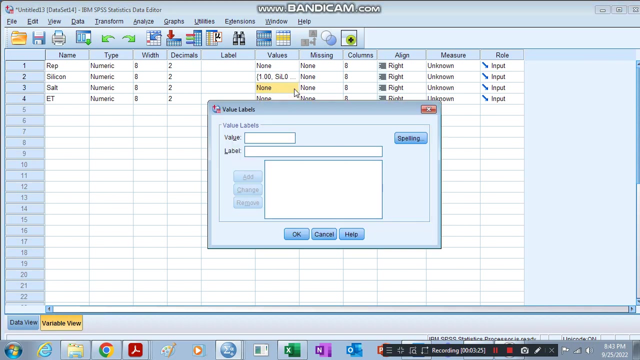 level. we have four salt levels each level in each silicon level, one, two, three, four salt level and we have, uh, the values of our dependent variable, which is evapotranspiration. then we have something to manage also here in variable view. so here for silicon and salts we need to write what represent what. for example one. 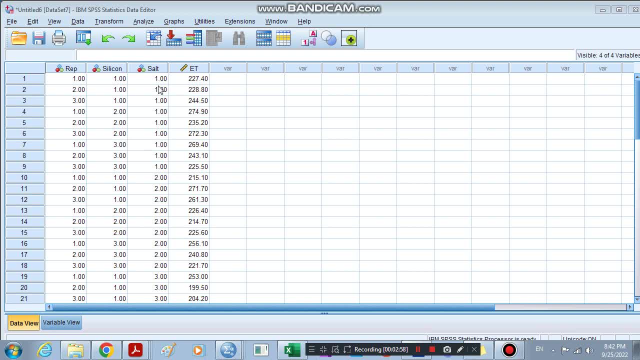 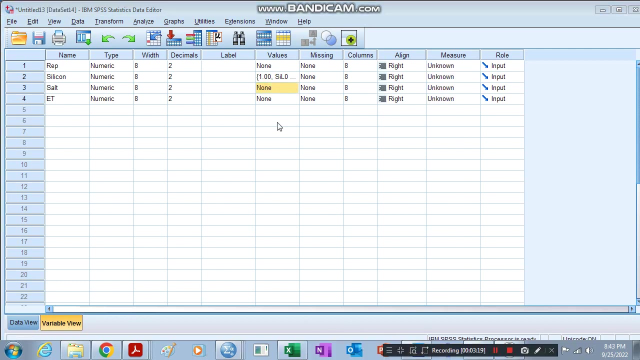 levels, each level in each silicon level one, two, three, four salt level and we have the values of our dependent variable, which is evapotranspiration. then we have something to manage also here in variable view. so here for silicon and salts we need to write what represent what. for example: 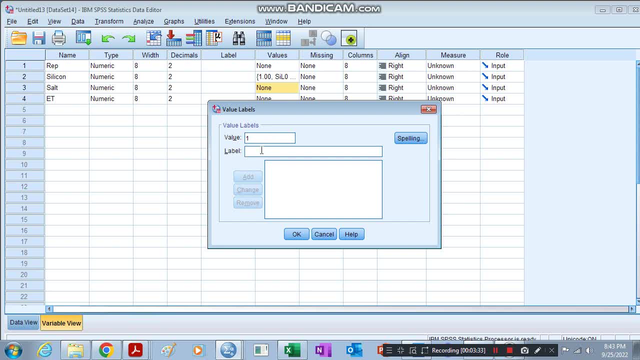 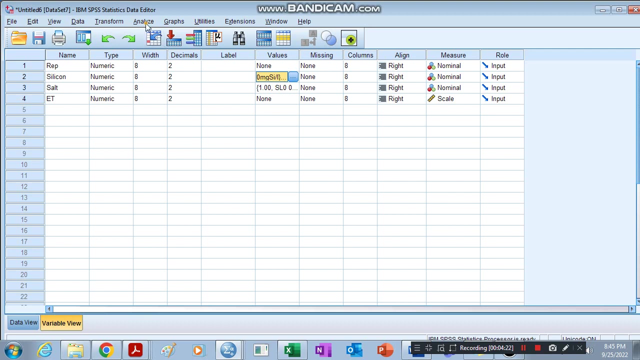 one in the data view represents for our salt level as salt level zero, which is zero point six. this is summits per meter odd, and two represents salt level one, which is one point six. this is techniques per meter. then, after writing the numbers which you represents different levels of silicon and salts. then we directly go to analyze parts. 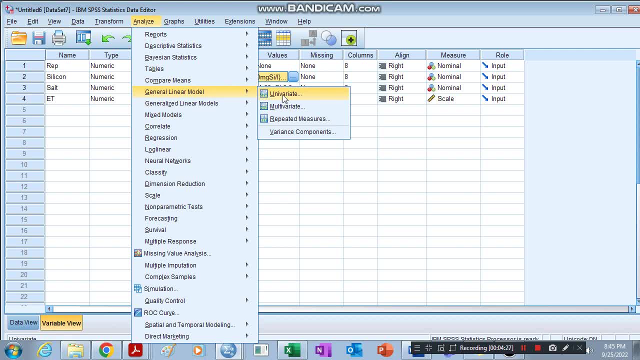 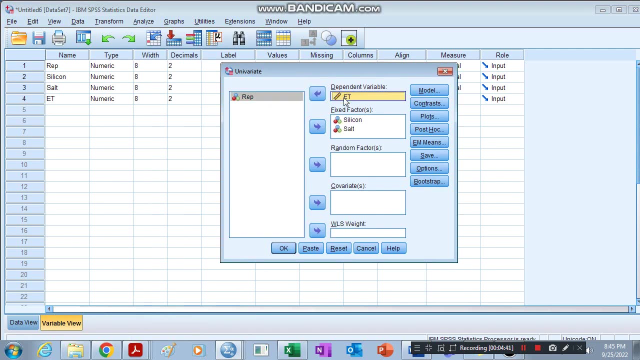 general lineal model model. then we go to universe univariate, because we have just one dependent variable which is evapotranspiration. then when you, we go to here, we found, we find it like this, then we just take our dependent variable to dependent variable box, our factors, which are, which has two: 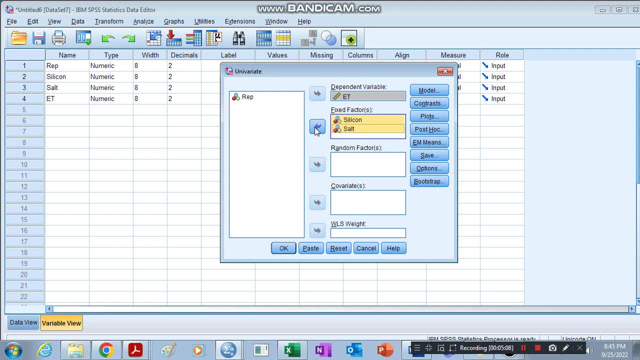 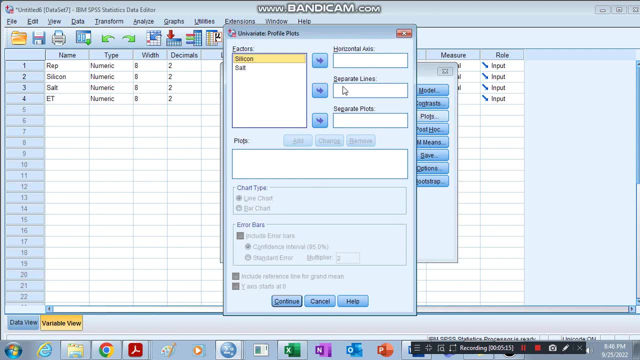 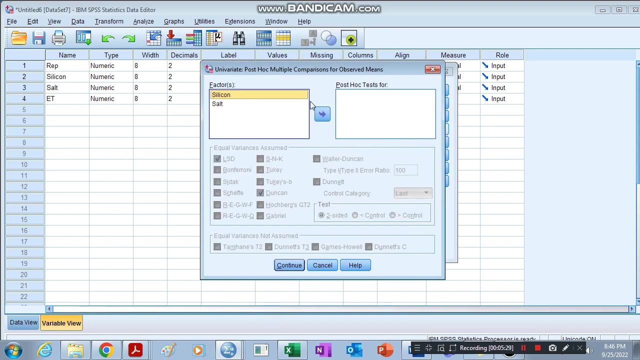 we. we have two factors: silicon and salt. we just put them in the fixed factor box. then we go to plots. we can put our salt factor in a horizontal axis, then the silicon in separate line, then add, continue. post hoc we select both of our factors. then we highlight lacd and duncan to taste. 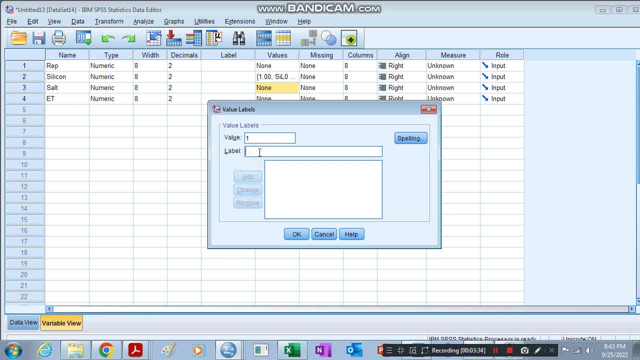 in the data view represents uh for our salt level. this is salt level zero, which is 0.6 decisiveness per meter add, and two represents salt level one, which is 1.6 decisiveness per meter add. then, after writing the numbers, which represents different levels of silicon and salts. 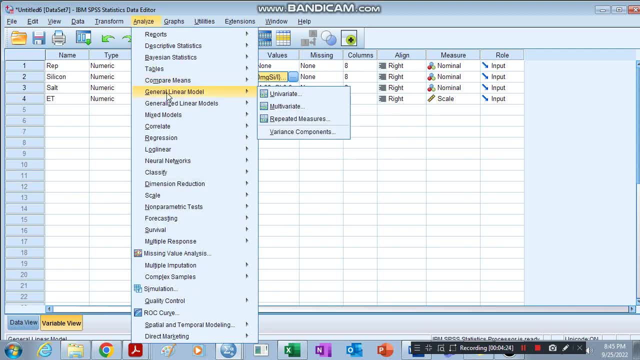 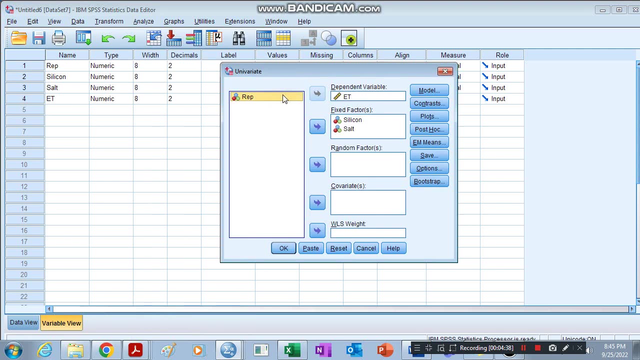 then we directly go to analyze parts, general lineal model model. then we go to universe univariate, because we have just one dependent variable which is evapotranspiration. then when we go to uh, here we found, we find it like this, then we just take our dependent variable to dependent variable box. 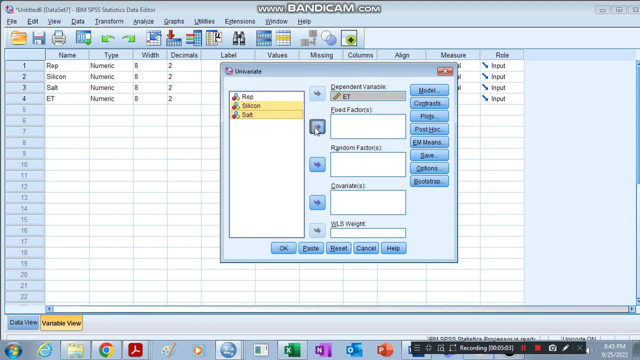 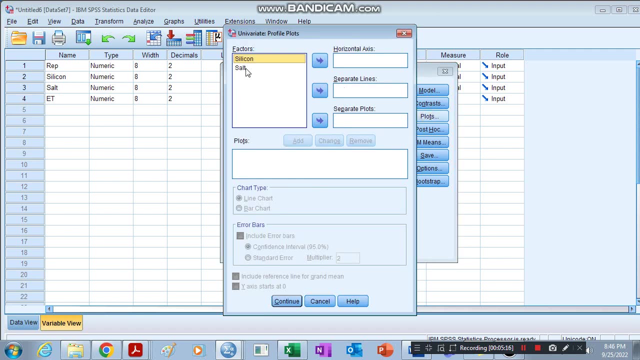 our factors, which are: which has two? we, we have two factors: silicon and salts. uh, so i can just reduce its level based on the number of blue s comfortable than the simples. i can reduce its number. factors silicon and salt: we just put them in the fixed factor box. then we go to plots. we can. 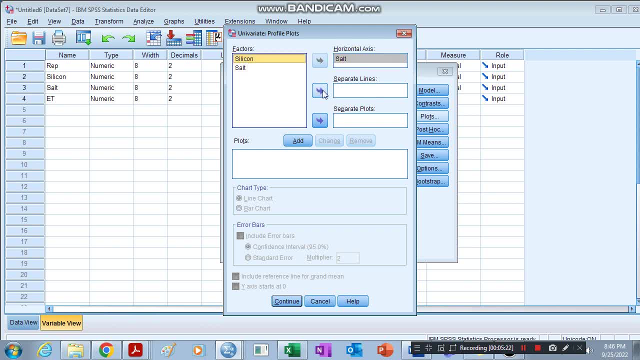 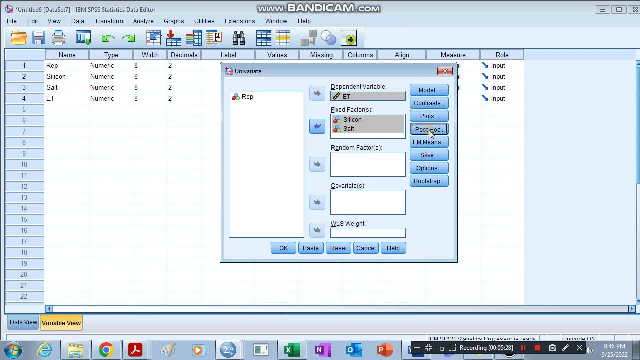 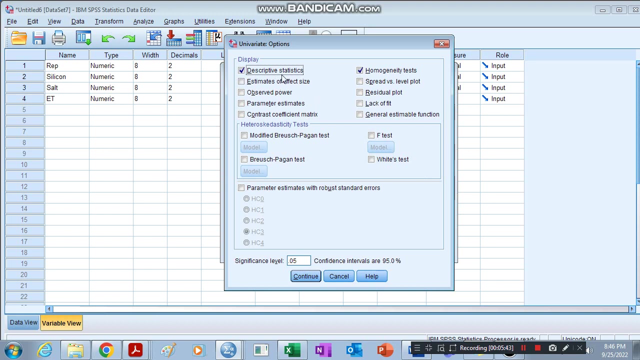 put our salt factor in a horizontal axis, then the silicon in separate line, then add continue post hoc. we select both of our factors, then we highlight lsd and duncan to taste. then we go to option menu. then descriptive statistics and homogeneity test has to be. 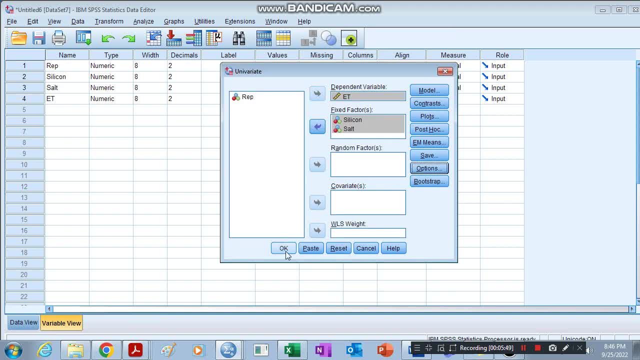 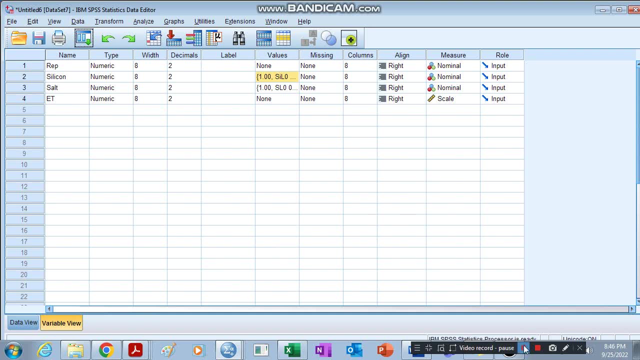 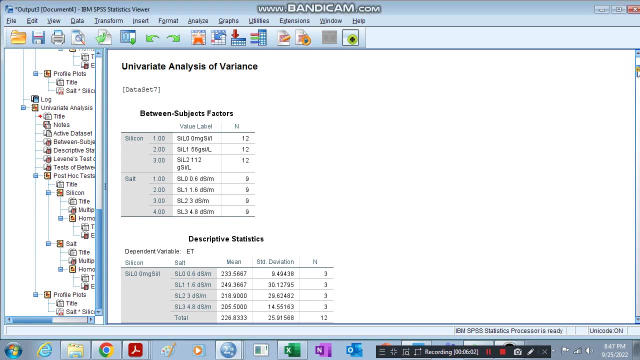 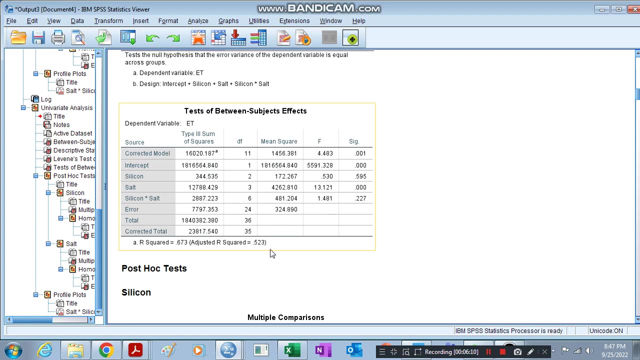 highlighted, then continue and we click on ok, we are now analyzing our experiment. then we go to uh, our output page. after analysis we directly go to tests of between subject effects. then we can see our two factors here. silicon, for example, has no any significant effects on our dependent. 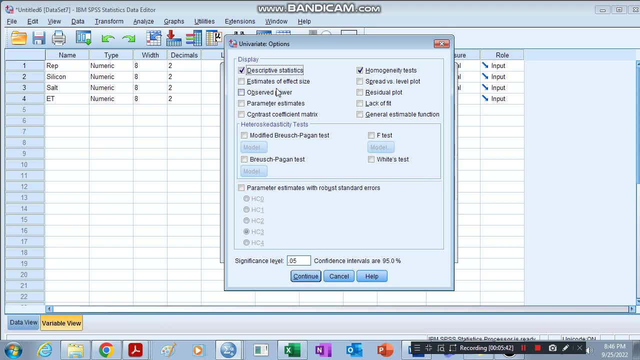 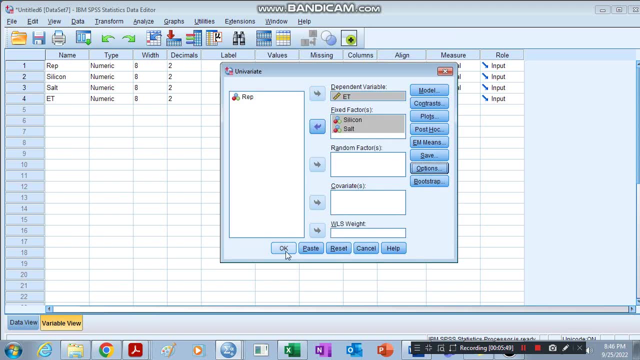 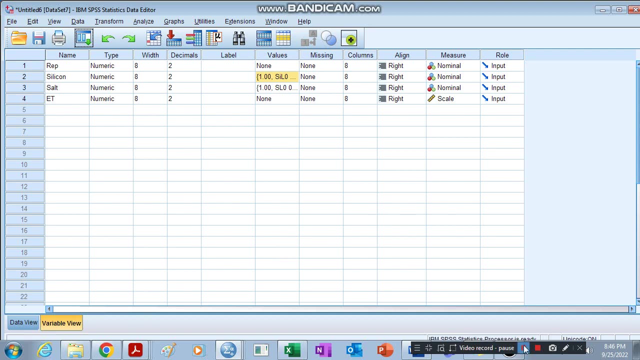 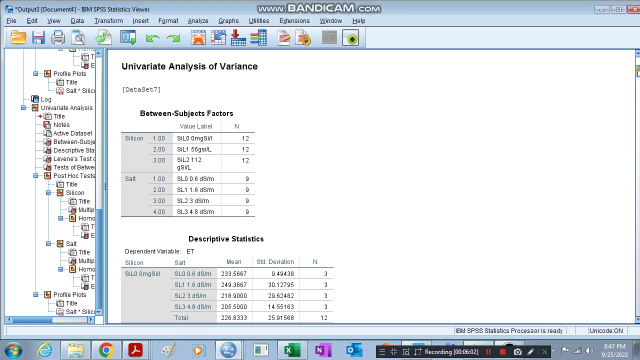 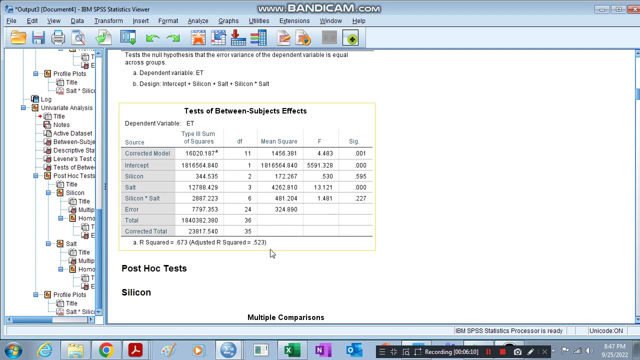 then we go to option menu. then descriptive statistics and homogeneity test has to be highlighted, then continue and we click on ok, we are now analyzing our experiment. then we go to our output page. after analysis we directly go to tests of between subject effects. then we can see our two factors here. silicon, for example, has no any significant effects. 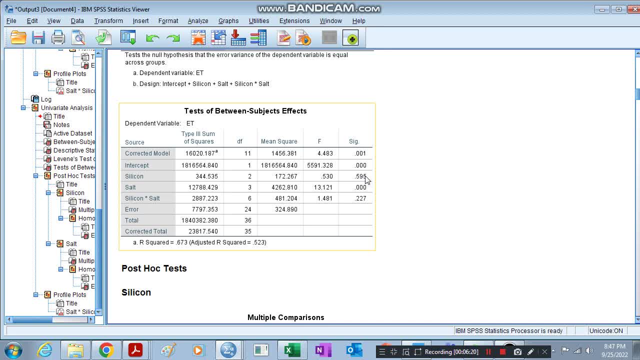 on our dependent variable, which is evapotranspiration, in. in order for it? uh to have a significant effect, it has, its number here has to be less than 0.05 uh, because our uh, we are testing uh by making our level of significance 0.05. 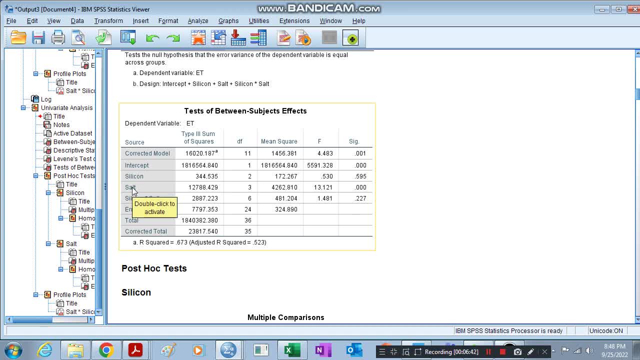 0.05. and when we come to the second factor, which is salt, it has significant effect because its value here, as you can see, is less than zero point, by far less than 0.05. so it has a significant effect on our dependent variable, which 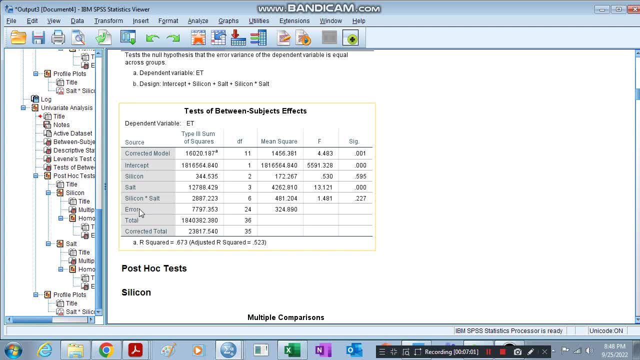 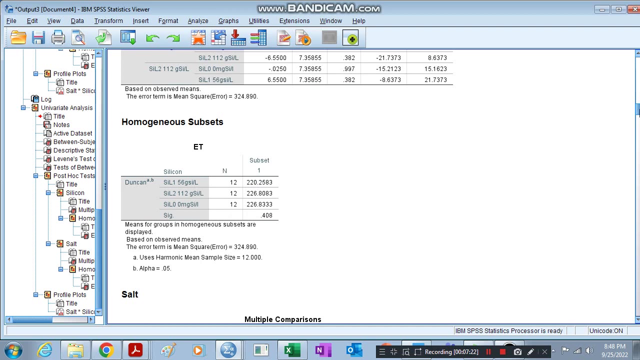 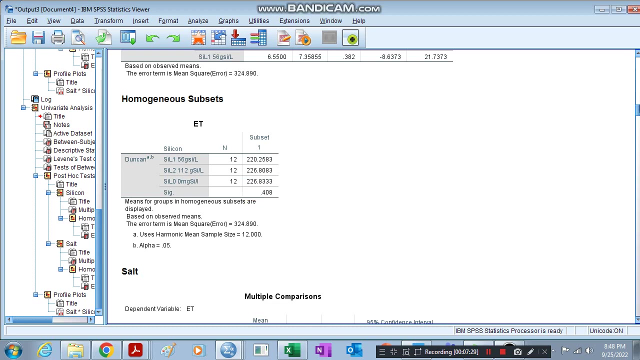 is evapotranspiration of the crop. when we see the interaction effect of this, both factors, these two factors, its interaction has no significant effect either. you can see here it's, it's not less than 0.05. so when we go to the homogeneity tests- the table here, it is for silicon. it has no effect, as we said. 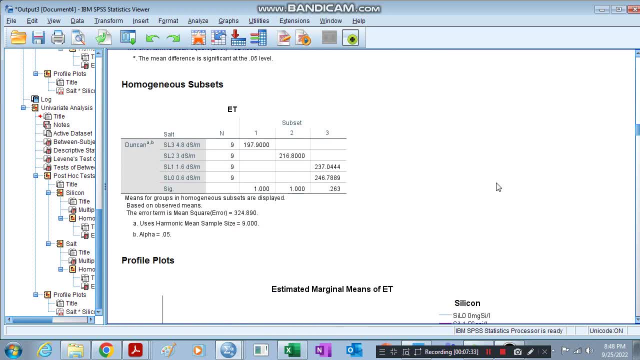 and for salt. it has an effect. you can put these values in your thesis or whatever and you can start, you know, explaining or interpreting the result. you can assign this a, this one also a, and the second to B and C, and then you can interpret in a. 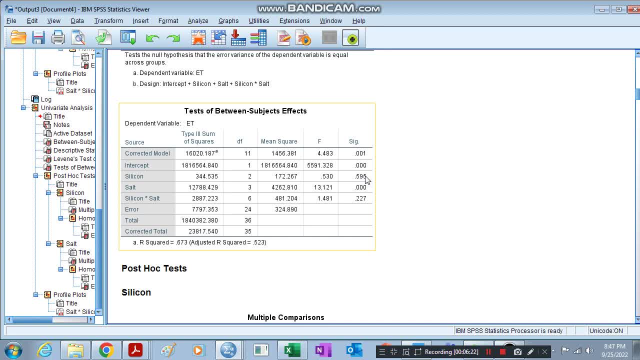 variable, which is evapotranspiration, in order for it to have a significant effect- it has, its number has to be less than 0.05. uh, because our uh, we are testing uh by making our level of significance 0.05. and when we come to the second factor, which is salt, it has a significant effect because its 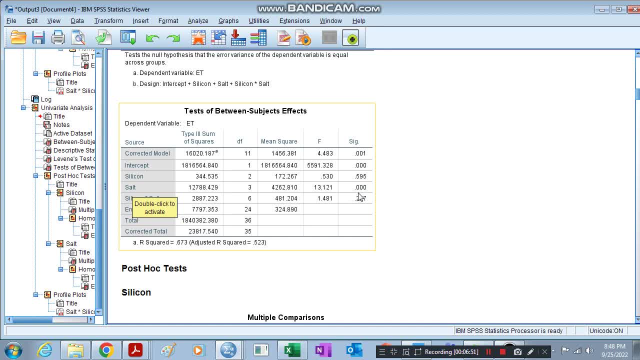 value here, as you can see, is less than zero points, by far less than 0.05. so it has a significant effect on our uh dependent variable. it has a significant effect on our dependent variable, which is evapotranspiration of the crop. when we see the interaction effect of this, both factors- 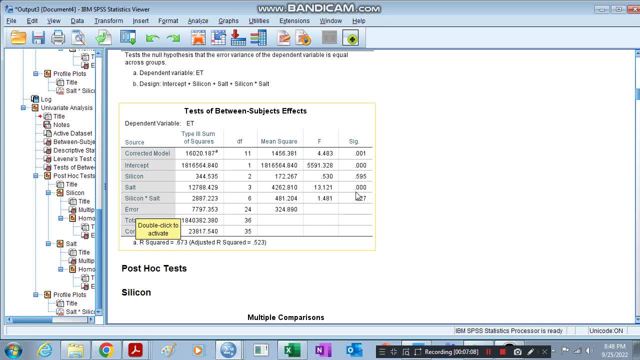 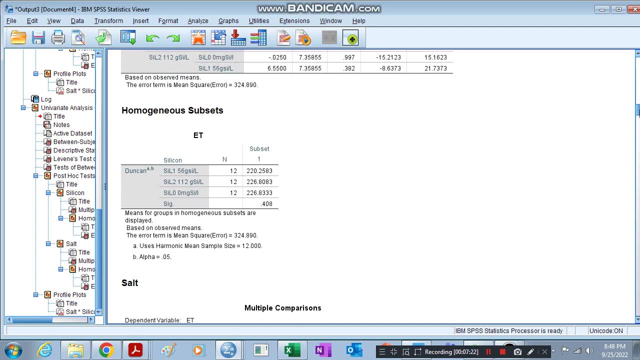 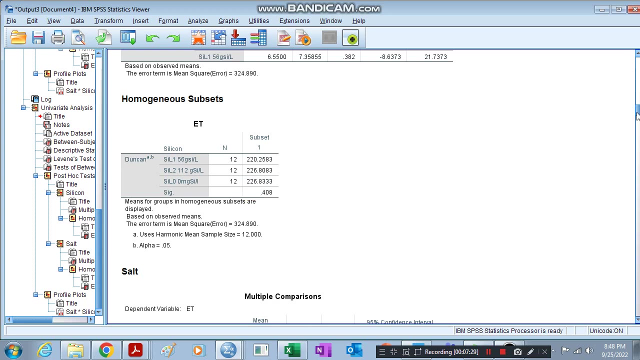 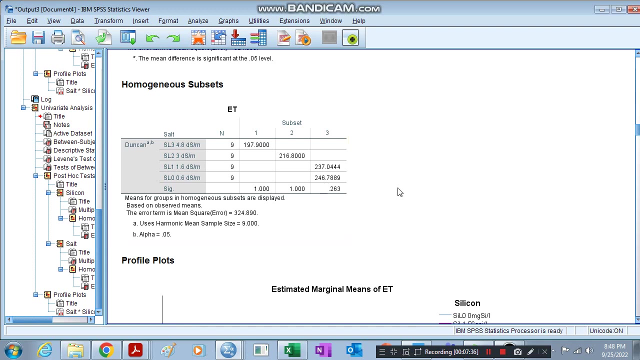 these two factors, its interaction has no significant effect either. you can see, here it's, it's not less than 0.05. so when we go to the homogeneity tests, the table here, it is for silicon effects, as we said, and for salt it has an effect. you can put these values, uh, in your thesis, or 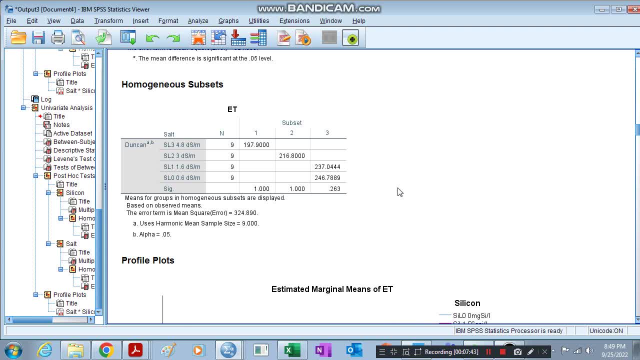 whatever, and you can start, you know, explaining or interpreting the result. you can assign this a, this one also a, and the second two b and c, and then you can interpret in a way that this value the, the third and fourth levels of salt, not the first and second of salt. 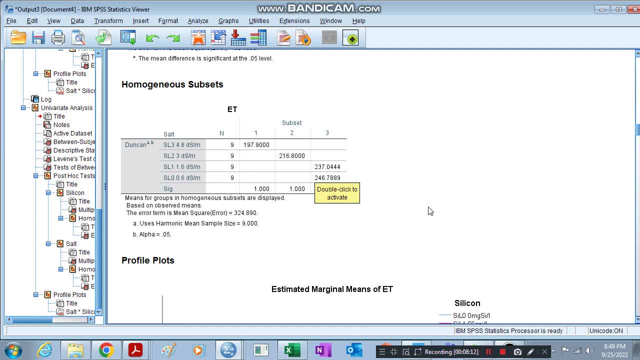 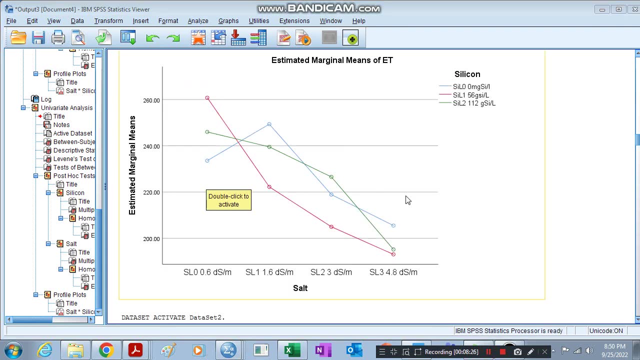 level has high, significantly high, value than the the rest of the salt levels. when it comes to evapotranspiration of the crop, we can interpret it like this: as you can see, this is the plots we found here in the output page. so it shows that as salt level increases, the evapotranspiration of